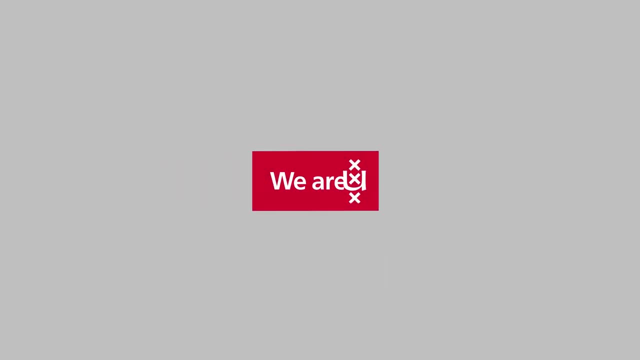 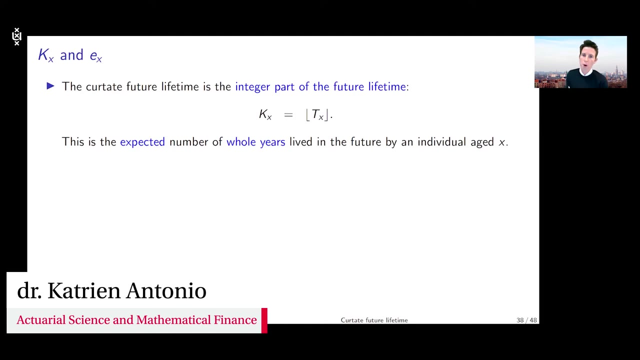 We're going to look at the integer part of the future lifetime random variable. So we're going to look. we're going to introduce a new random variable denoted with kx, and kx is the so-called floor function applied to tx. 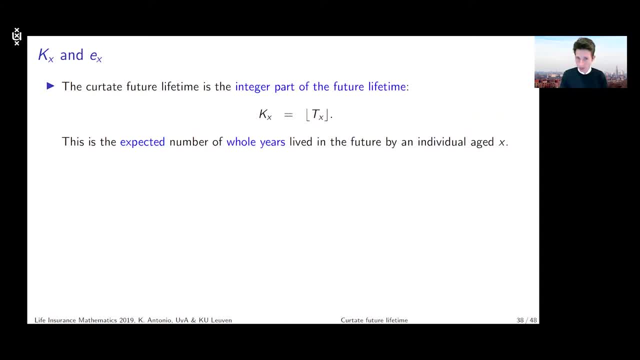 So tx is a continuous random variable so it can take positive outcomes in continuous time And with the kx we're going to look at the integer part of my future lifetime. So the kx is a discrete random variable. It's the expected number of whole years. 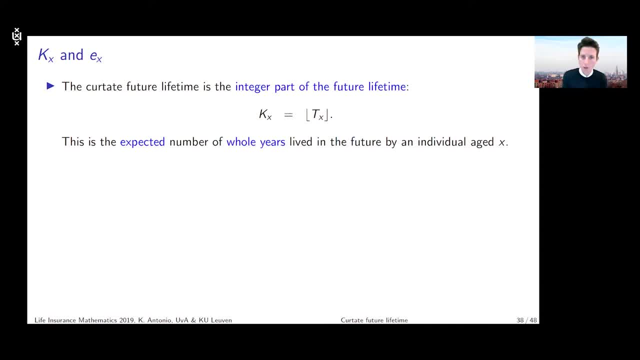 If you take the expected value of kx, you're looking at the expected number of whole years that is lived in the future by an individual age. And why is that interesting to look into? Because often an insurance product will pay out at the beginning of the year or at the 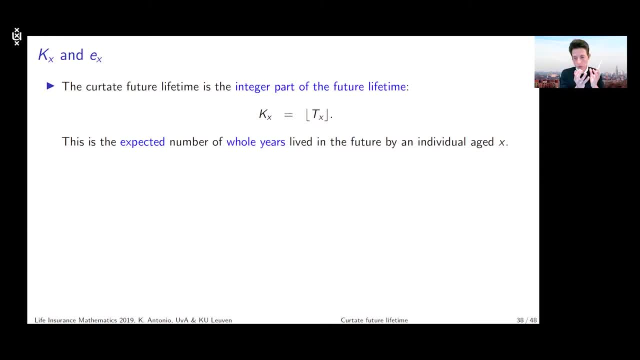 beginning of the month or something, And if you look at a product that pays out at the beginning of the year, then the number of payments that you can expect for this individual to take place will be captured by the expected value of this kx. 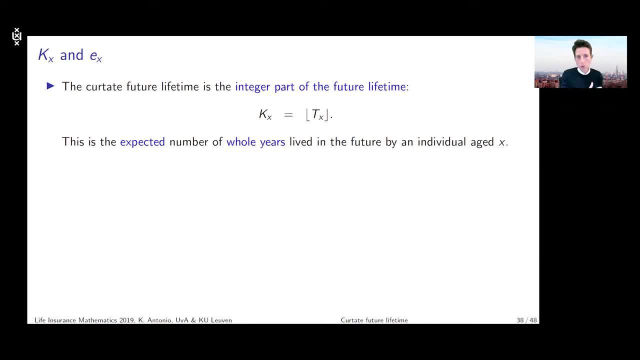 Because then you need to know how many whole years will my individual continue to live in the future, right? So don't worry yet about these actuarial use cases. yet that will come later on. So for now, just keep in mind there is this curted future lifetime. it's denoted with 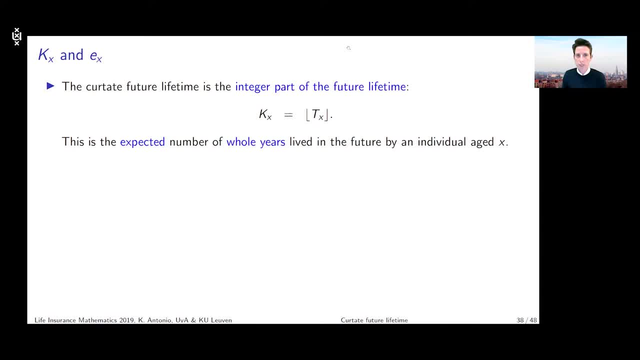 kx and it's the floor function applied to tx. So what I'll try to do with you is try to make sense of the probability function Of kx. So I'm going to wonder: what is the probability that kx is equal to k? 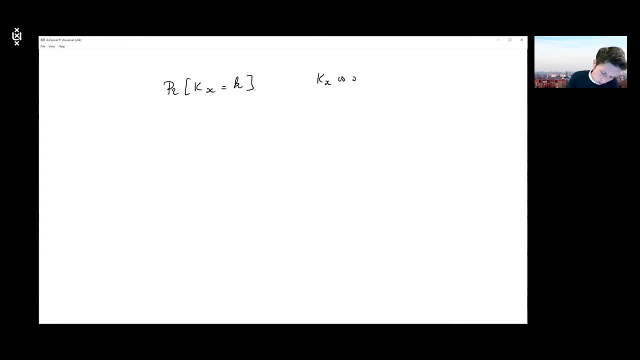 So kx is a discrete, random variable and it's taking positive values. So if I want to say something about its distribution, then I need to find an expression for what is the probability that kx takes the value k. Now, if kx takes the value k, then that means: 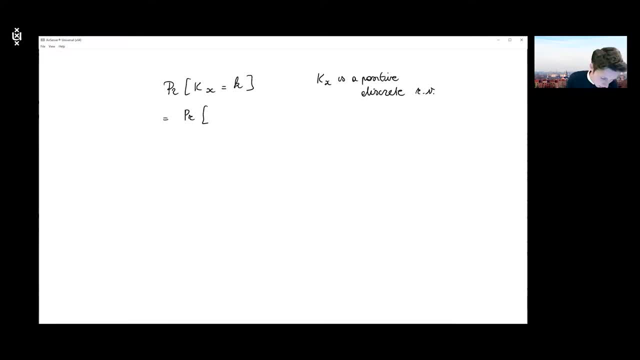 Because of the definition- Okay, The definition- of the floor function, that my corresponding tx will take a value between k and k plus one right. Because, if I would draw my timeline, I'm looking at an individual who is x year old at time. 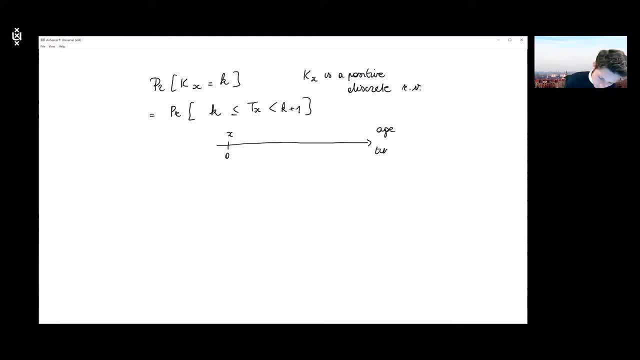 zero. So this is h and this is time, And I want to know what is the probability that this individual will die between hx plus k and k And hx plus k plus one. So I want to know what is the probability that I'm in here. 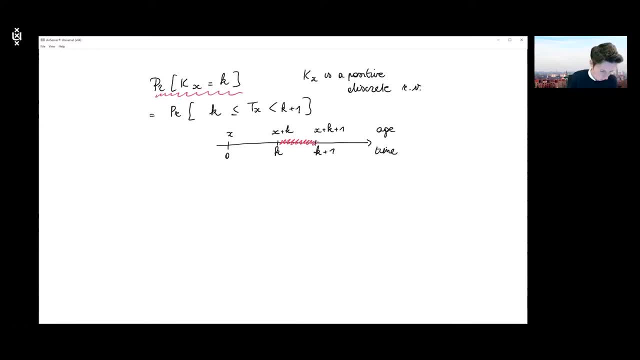 That's what this probability is capturing. Okay, So I need to know how to express this. So, if you look at the timeline, you could say: well, using our previously introduced notation, that is a deferred probability of dying, Namely, you need to survive k years. 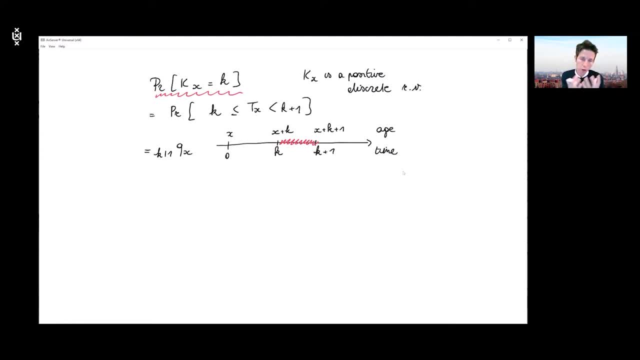 And then, after reaching hx plus k, I want to know, I want to know what's the probability that you will die within one year from there. So one way way to rewrite this thing is by saying: it's the probability to survive k years minus the probability to survive k plus one years. 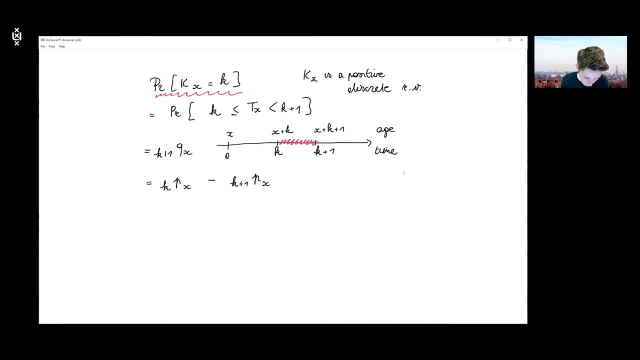 And if you don't see that immediately, once again, I would recommend you to picture this on the line. So if you look at the probability k px, That's the probability To go Beyond H X plus X plus k. 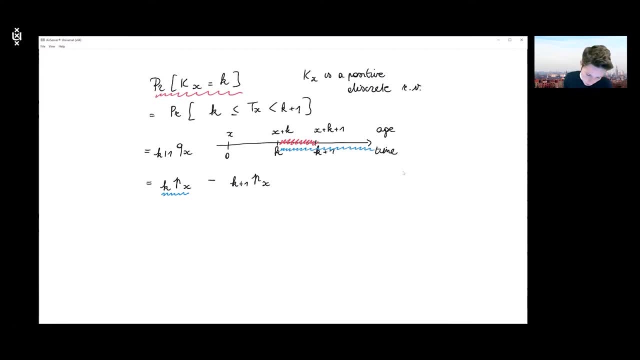 Right And if you subtract the probability To go beyond H, X plus k Plus one Right. So if you start from the blue guy, you subtract the green guy, then you're left with the area in red Right. 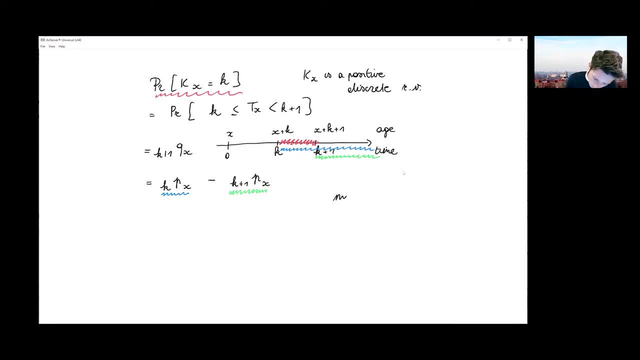 So that's what we want to do Now. we learned something powerful on Monday, and that was our multiplication rule. So the multiplication rule Allows us to say that k plus one px is equal to k px multiplied with p x plus k. If you survive another k plus one years, then you first need to survive k years. 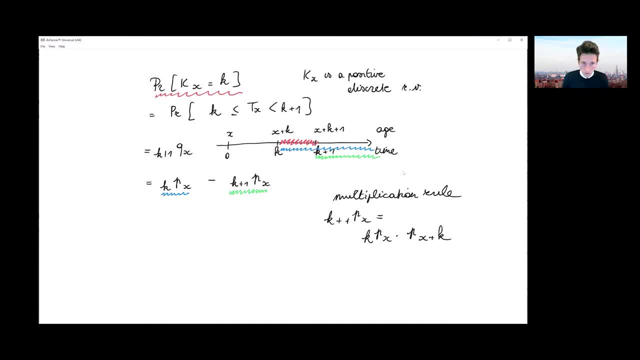 You reach h x plus k and then you need to survive another year. So plugging in this guy into the expression that we have over here will retrieve k px minus k px, K px multiplied with p x plus k. I'm going to manipulate this expression and I'll retrieve something like this: 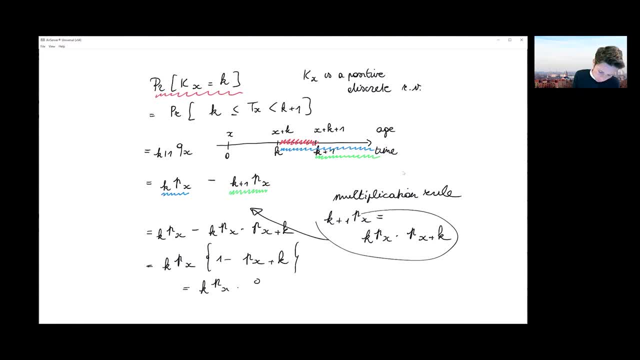 Which I can rewrite them as k px multiplied with q x plus k. So this gives me in quite a handy format the probability function of my curted future lifetime random variable of my k x. Yeah, So the probability that k x is equal to k, you can construct it by saying you first have 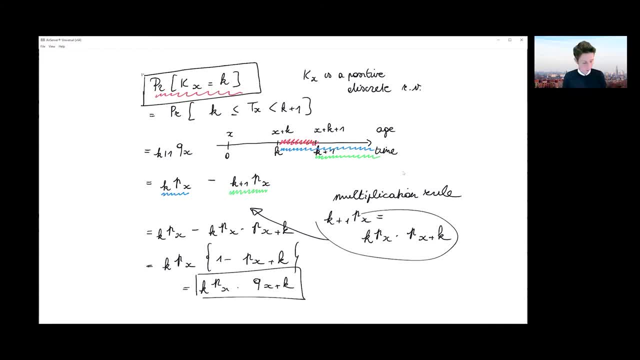 to survive k years and then you'll die within one year from reaching that h. Now, having this k x and its distribution, we're ready to calculate the expected value of the k x, and that will be the curted future. expected future lifetime of an x year old. 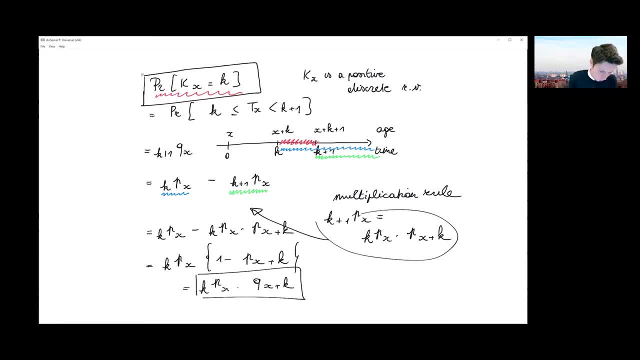 So let's do that one together as well, as a final step for this chapter. So I'm now interested in What is this? What is the expected value of k x? So let's move on with calculating the expected value of k x. 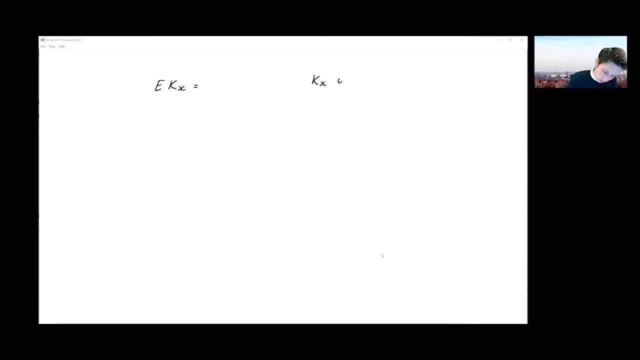 So k x is a discrete random variable. So what you then have to keep in mind is the way how you learned to calculate the expected value of a discrete random variable. So you did that by taking a sum over all possible outcomes, k, that this random variable can take. 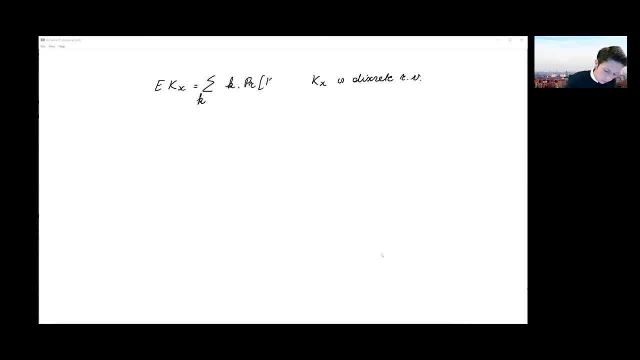 And you do. You multiply it with the probability that your discrete random variable is going to take this value Right. So this is, with the sum construction, the expected value of a discrete random value. So what we learned now is a way to express this probability function for the k x. 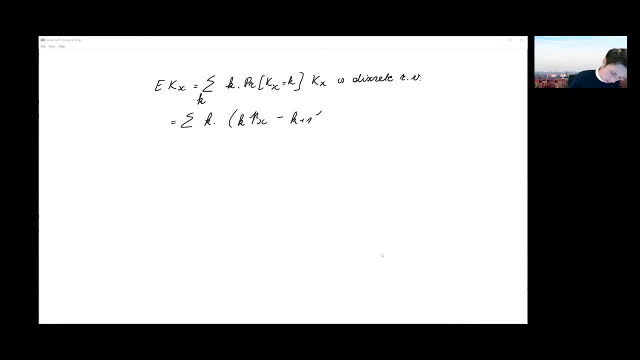 So that was k p x minus k plus one p x, and the k can run here from zero to, Let's say, plus infinity. plus infinity, because the first value that the current, future lifetime, lifetime variable can take is zero. right, That means that you die within one year from now. 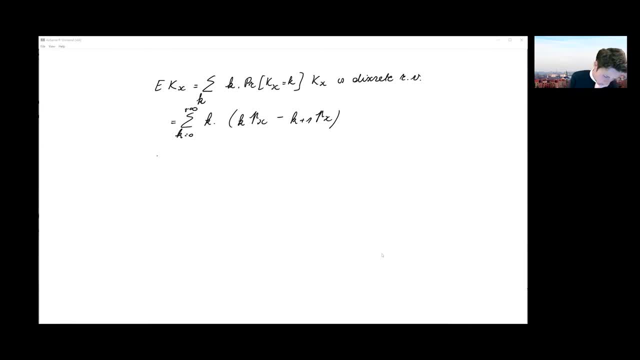 So if we're going to manipulate this expression, what we then see is that if k is equal to zero, then this term drops, because k is zero, and this will lead to no contribution. If k is equal to one, then I have a contribution one p x minus two. 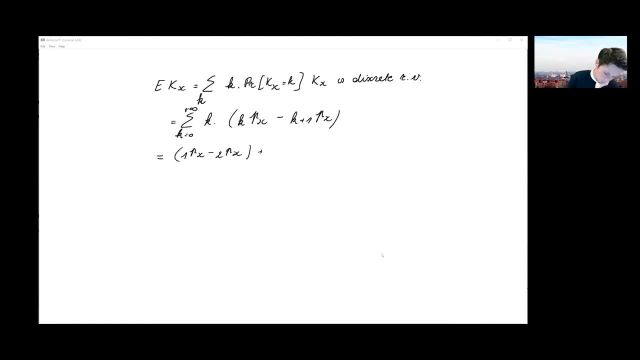 Two p x. If k is equal to two, then I'm going to contribution two times two p x minus three p x, and so on and so forth. right? So if I work out this expression, what I will see then is that a lot of the terms here are. 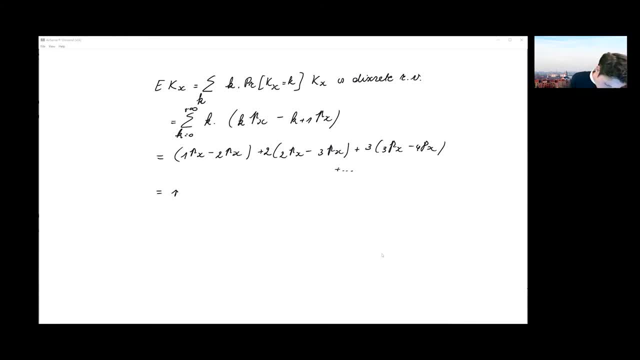 going to drop and I will be left with one p x, One p x and then I'll get two p x. Where do I get the two p x? Because I've got two times two p x minus two p x over here, and that continues in the same. 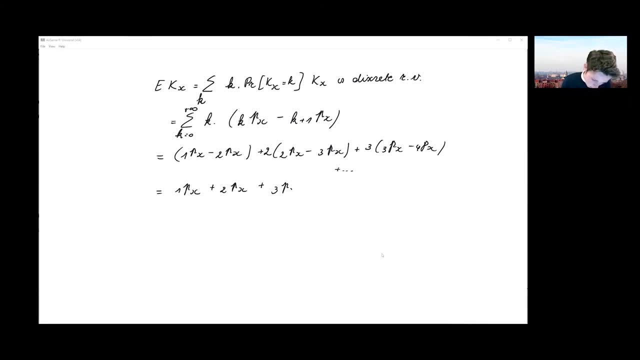 way. So that is, I've got a three p x and so on and so forth. So in the end I can express my expected value as the sum of k p x, and I'll be very careful where the k starts from zero. 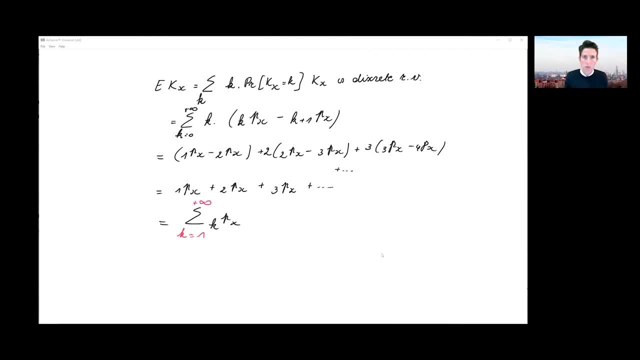 It starts from one and goes to plus infinity. So that is the expression that I have for my curted future lifetime and that's easy to calculate. That's the sum of my k, p, x's, The only comment when you're using this expression. so be very careful that you need to start. 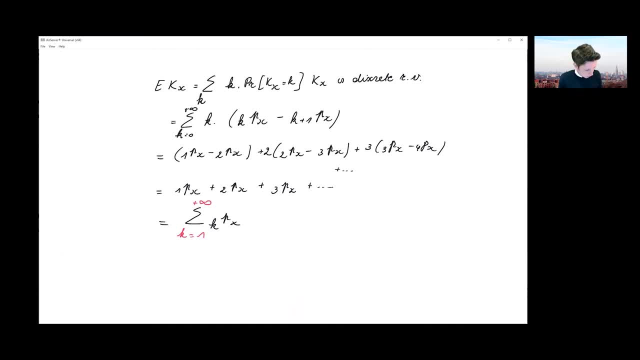 with k from one. Now, one of the things we often do is to build a connection between this Curted future lifetime, So the expected value of k- x, and the original complete future lifetime, The expected value of t- x, and that's something we often want to do. 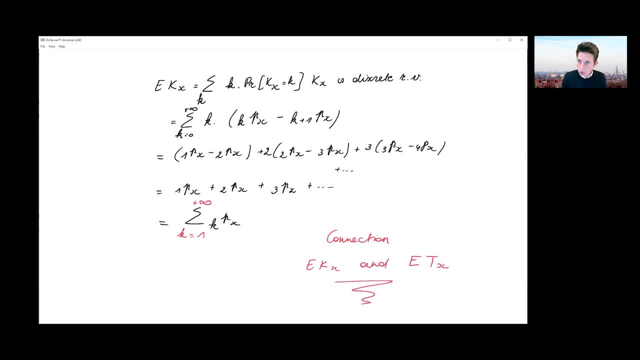 So let's take that as a last step. I'm going to start from the complete future lifetime random variable t x and I'm going to start from its expected value, which I know from what we learned So far that I need to calculate as the integral from zero to plus infinity of t, p, x, dt. 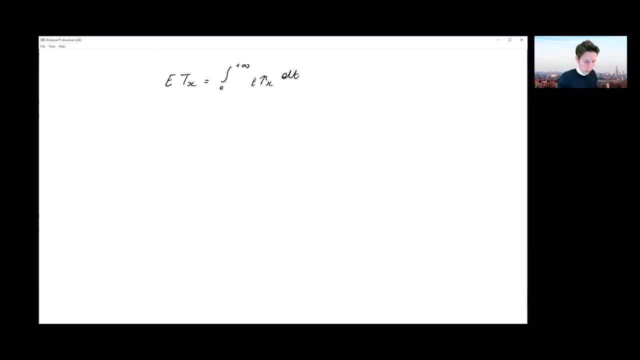 So that's in continuous time, right? So there you're using the t p x, where t can take a positive value in continuous time. So one way to approach this is by splitting this integral into intervals of length: one year. So then I go from zero to one, from one to two, from two to three. 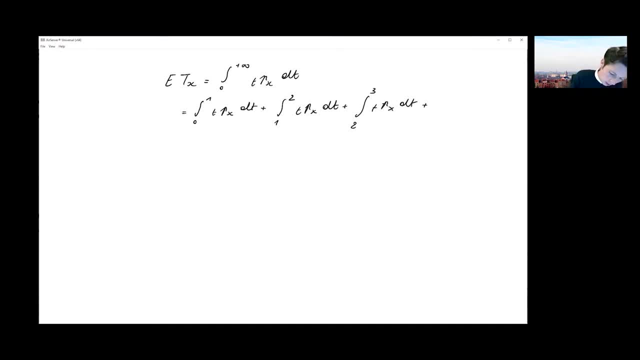 Etc. Okay, So that's one way to look at it, and a more elegant or a more compact way to write that mathematically would then be to write it down as a sum that goes from zero to plus infinity of the integral, from j to j plus one. 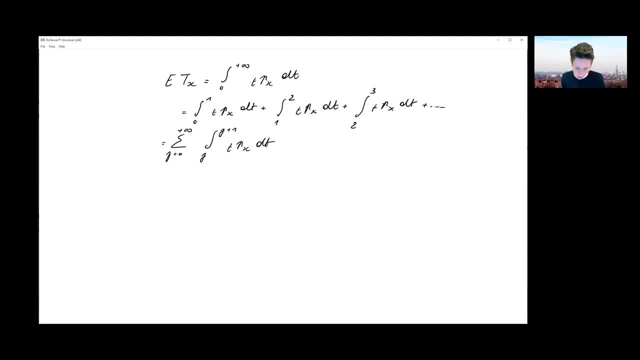 And then I look at t, p, x, dt. So that's exactly the same as start with j equals zero, and take j equals one, et cetera, et cetera. So you may recall from from other courses that if you look at this type of integral, 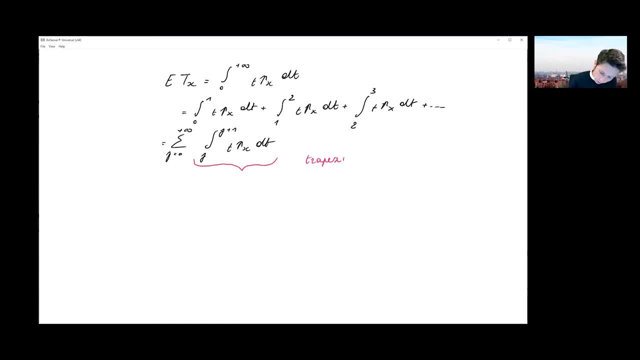 you can approximate it using the trapezium rule, And that's something you should not know for this course, but let's just apply it here. If you look at it, we can say: this is approximately equal to the sum over j of j p, x plus j plus. 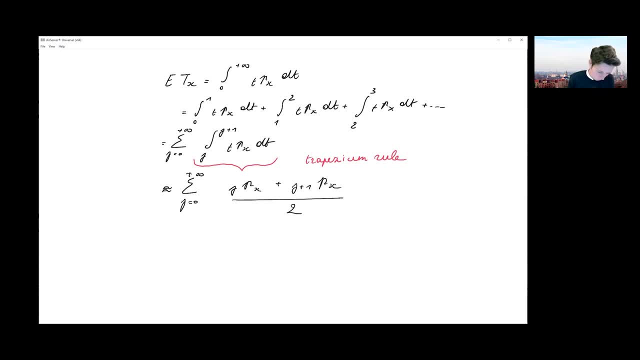 one p x divided by two, Okay, Okay, And what I can then do is then I can write this in full and I could say: well, that's zero p x plus one p x divided by two, And then I'll go on with one p x plus two p x divided by two, and so on and so forth. 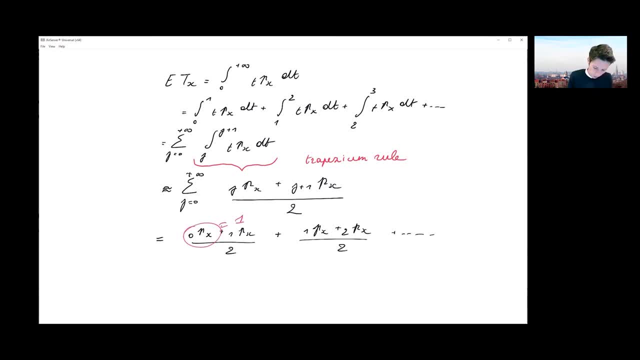 And this zero p x, that's equal to one right. So if I work out this expression, I'll get one over two plus one p x divided by two plus one p x. So that's one over two plus one p x divided by two plus two p x divided by divided by two. 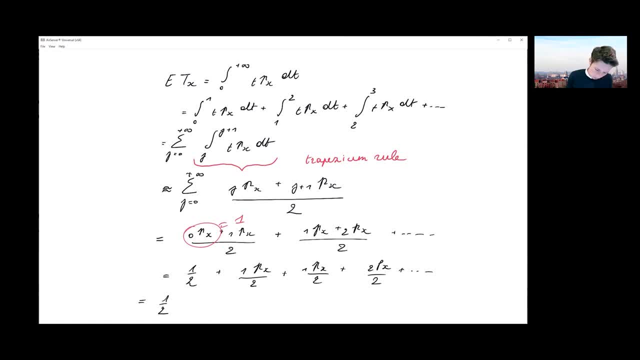 and so on and so forth. So in the end you'll find the following connection: It's one over two and then the sum over k, starting from one of k, p, x. And why is this so interesting? Because it shows us that the connection between the two kinds of life expectancies that we